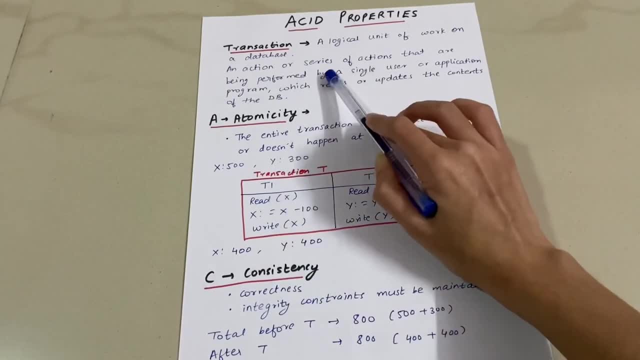 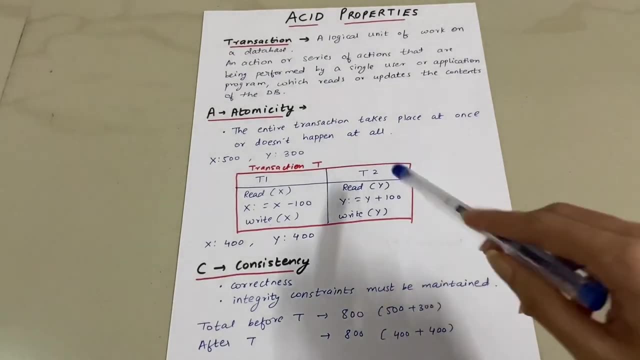 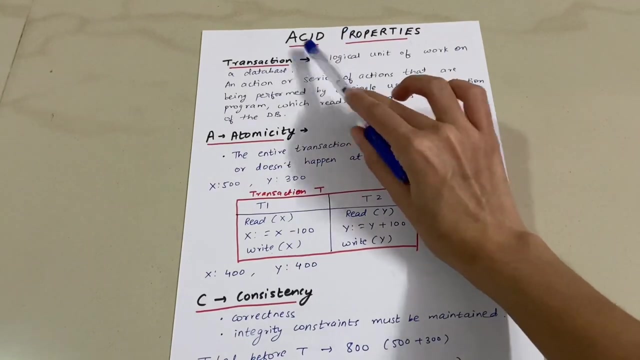 are changing the value in DB, So a transaction will be considered as this only, like a series of updates or all these things. So this is what transaction is, And a transaction must follow ACID properties. So ACID stands for A stands for Atomicity, C stands for Consistency. 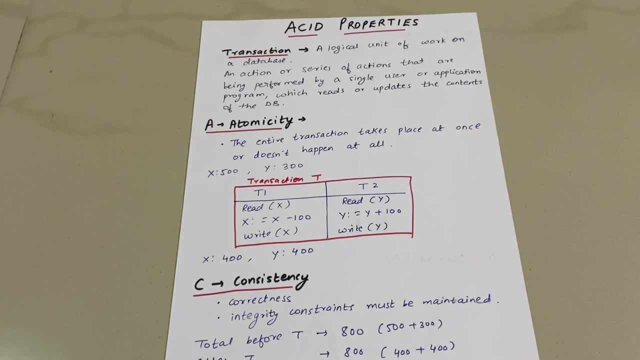 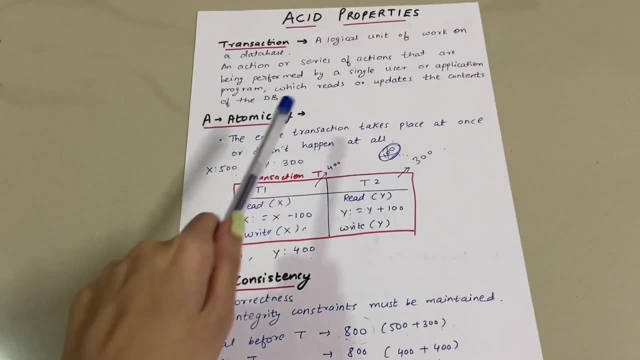 I stands for Isolation and D stands for Durability. Now, in this means that we will put two transactions one by one, So atomicity is the first property, So which means the entire transaction takes place at at- once or doesn't happen at all. 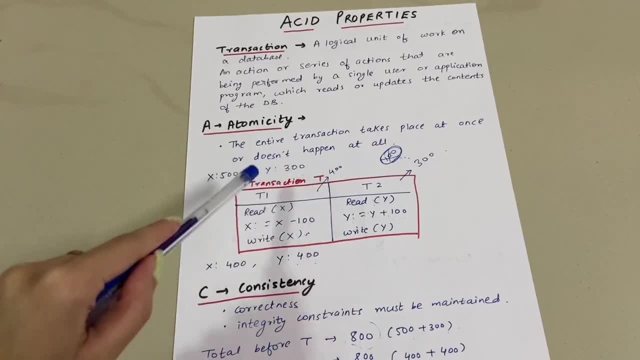 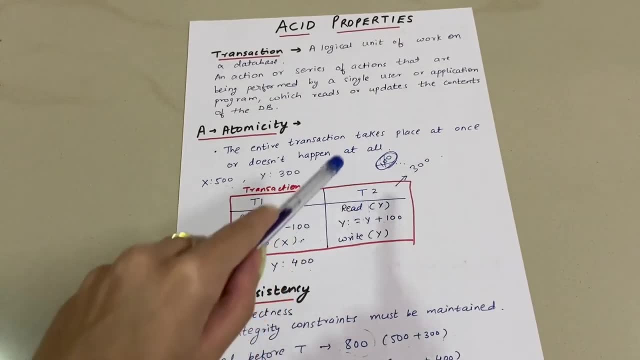 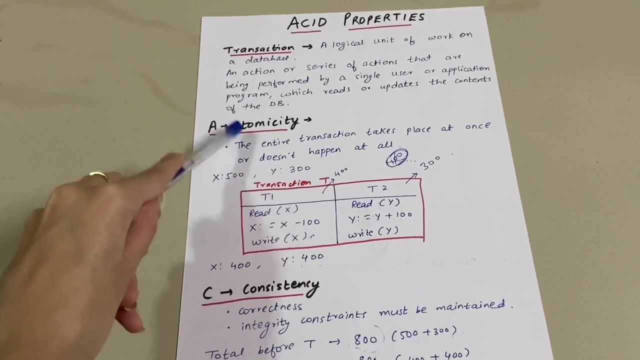 So let's consider this transaction, this whole transaction T, which consists of T1 and T2.. So in T1, money is being deducted from X and in T2, money is added in Y. So this is what the whole transaction T means, So that T means the whole transaction should. 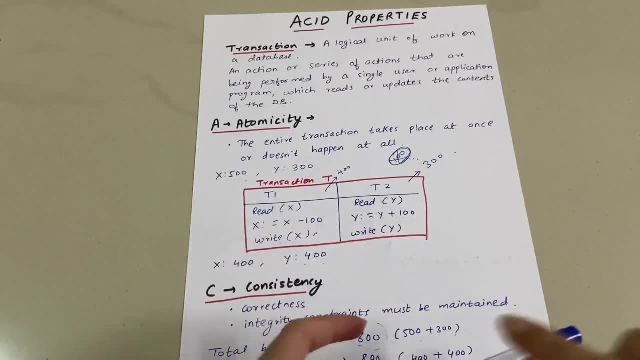 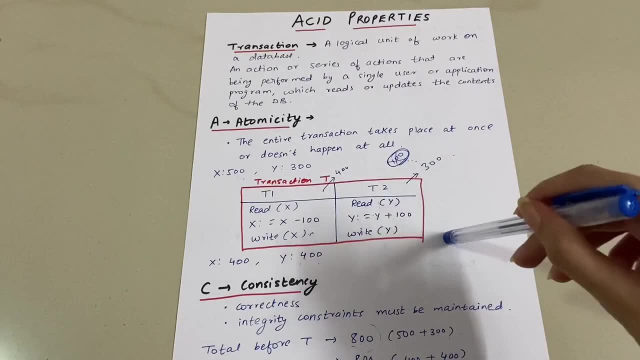 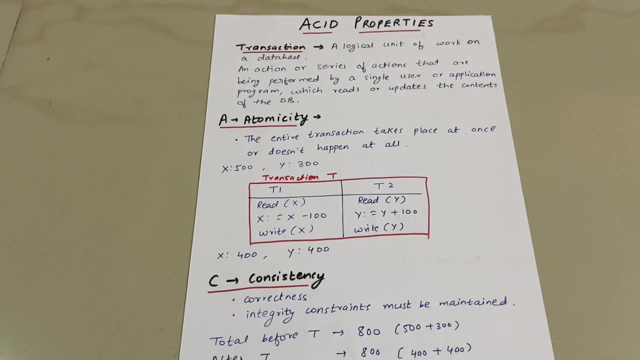 occur at once should be executed at once. if there is a system failure in between- in between, it will not be committed. either the entire transaction is to take place, and only then it will be committed, or if there is a system failure in between, it will be aborted. so, for example, the system fails after the 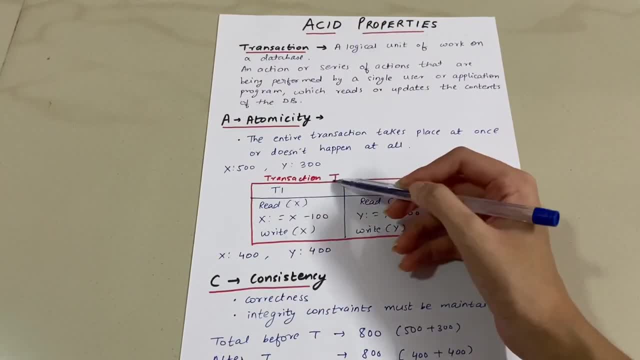 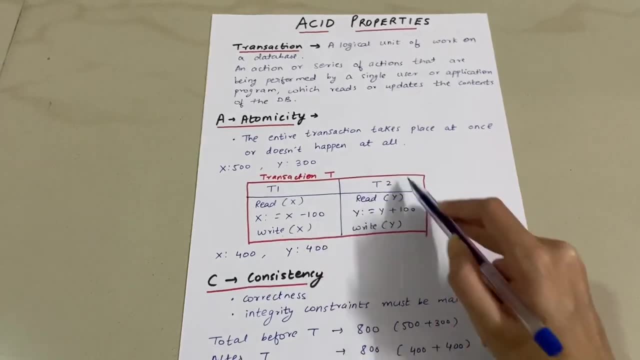 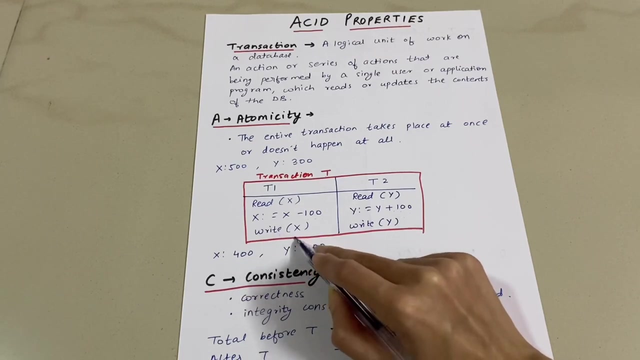 transaction of t1, so T is considered- is consistent of t1 and t2 transaction. so first t1 transaction will occur and then t2 will occur. so in case t1, if the system fails, after t1 and and before t2, so after t1 and before t2 if it fails. 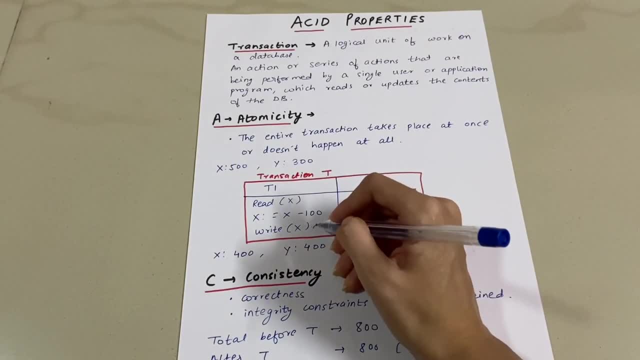 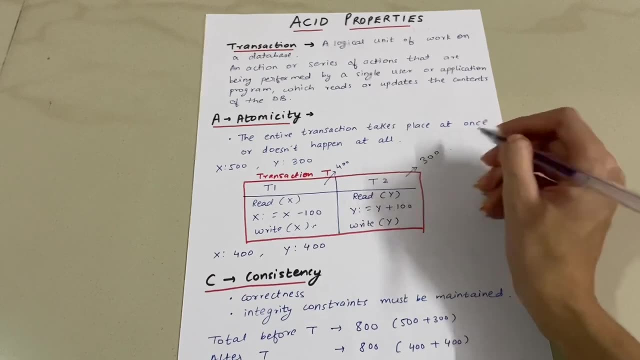 what will happen is this: from your, from X, money will be deducted. okay, 400, this will become 400, but Y will still have the same value, which is 300. so here there is a loss of hundred rupees. so this is the loss of hundred rupees. so 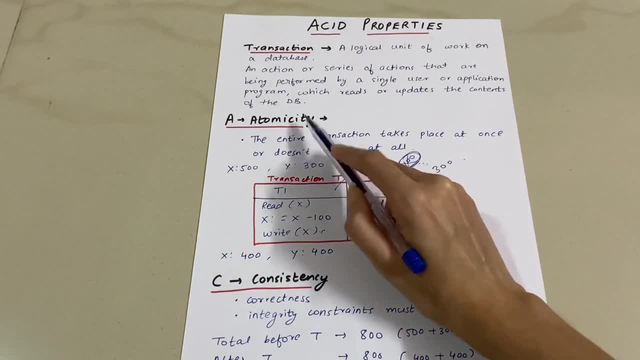 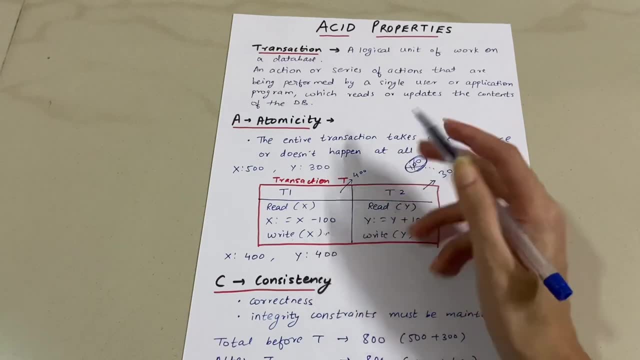 this is the loss of hundred rupees. so this is the loss of hundred rupees. so this is inconsistent data. so hence we need atomicity, which means either the full transaction will take place- there is no midway- you are the partially, partially transaction cannot be executed, either the full transaction will be. 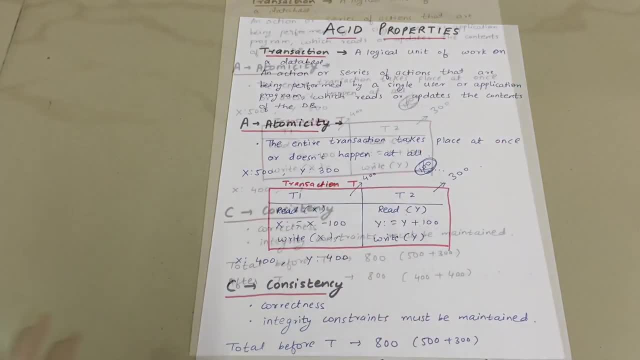 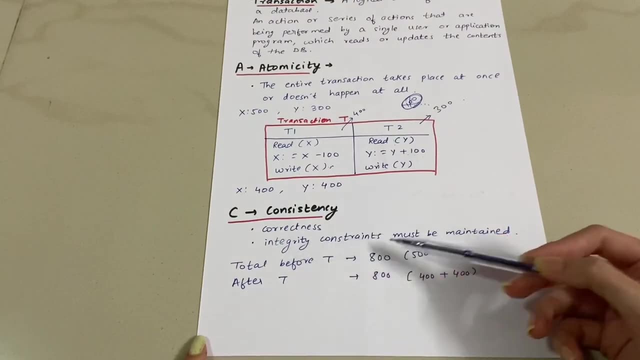 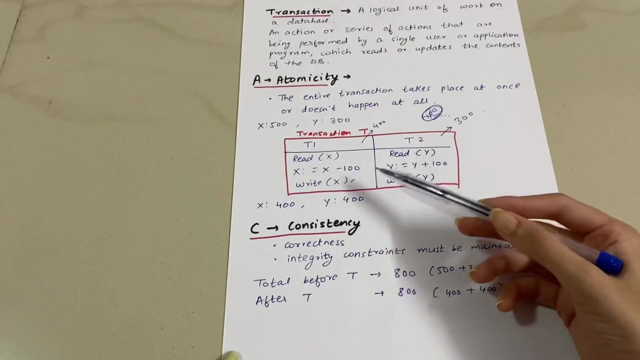 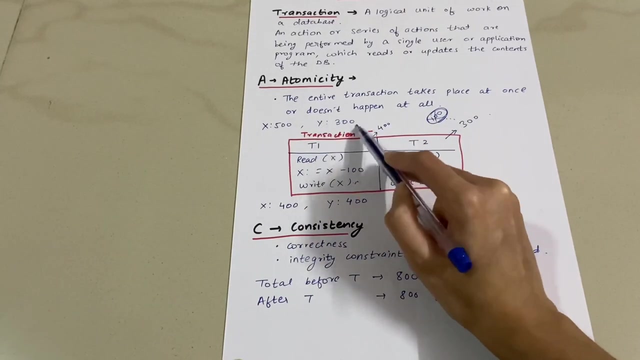 executed or it will not be executed at all. now, second property is consistency. consistency means correctness, so basically, integrity constraints must be maintained. so the amount before the transaction and after transaction should be same. now what that means is now, before transaction, as I had considered, X will have 500 rupees and Y will have 300 rupees. okay, okay, which is what is the 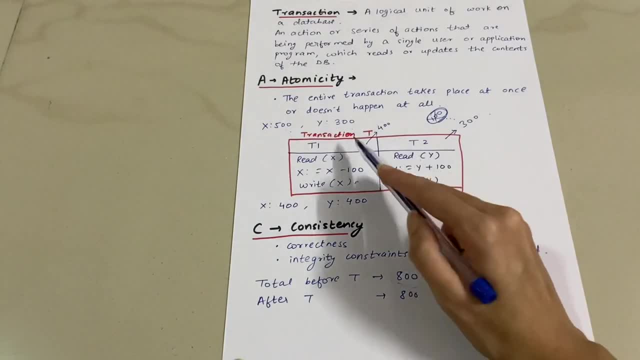 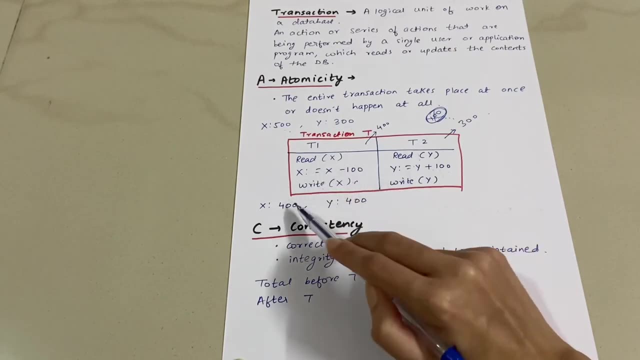 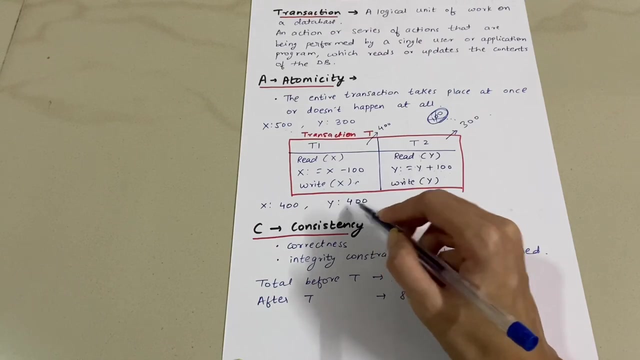 total of this: 500 plus 300, 800 and after, after the transaction, after money has been deducted from X. so X will become 500 minus 100, which is 400, and Y will become what? what was Y? 300? so 300 plus 1 400. so 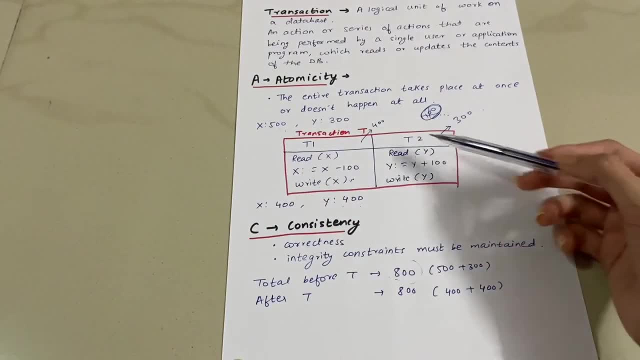 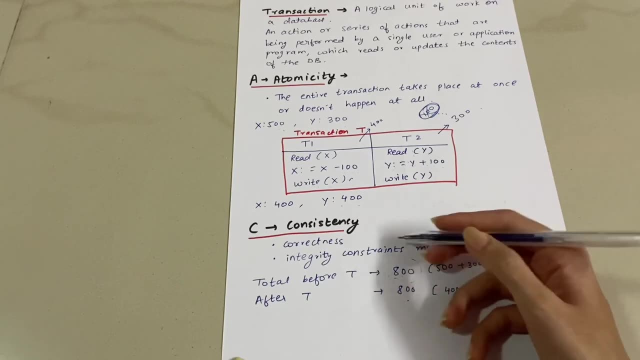 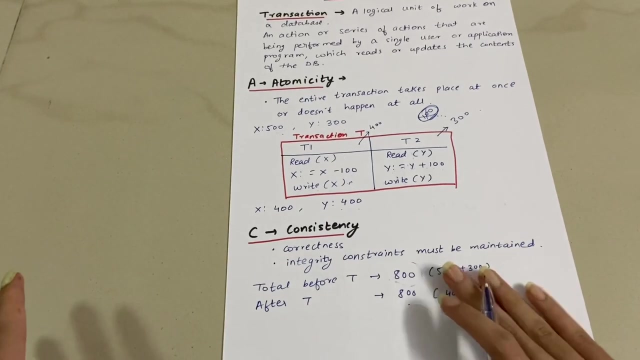 after the transaction: after the transaction T is executed, we have 400 plus 400, which is 800. so this is what consistency means: the total money should be correct, should be same. so correctness, the integrity constraints must be maintained. that is what consistency deals with. now, a third property is 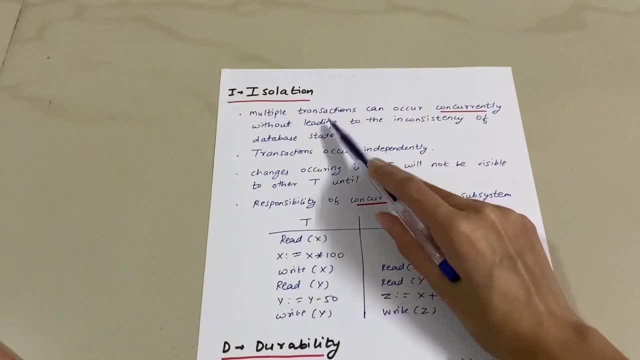 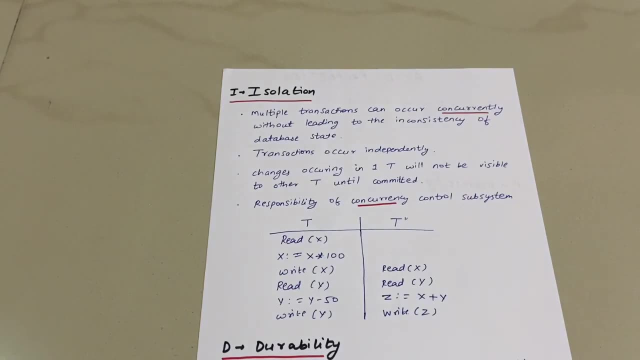 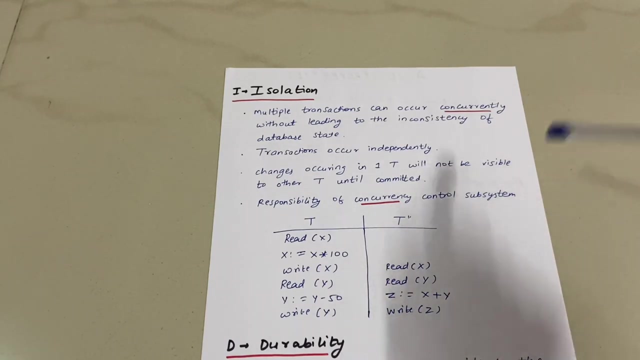 isolation. now what this means: multiple transactions can occur concurrently without leading to the inconsistency of the database. state now what this means is if you, if you take the example of a banking system, at a single time, a lot of customers are accessing it, so multiple transactions can occur concurrently. okay. 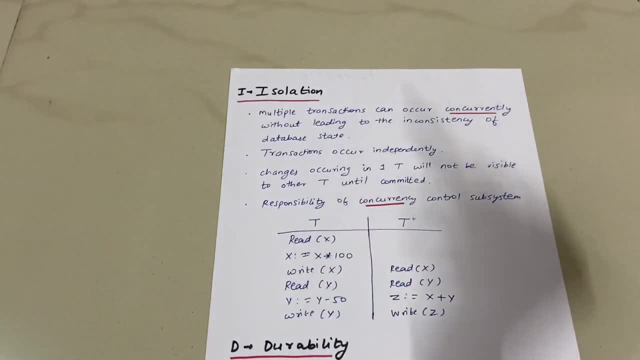 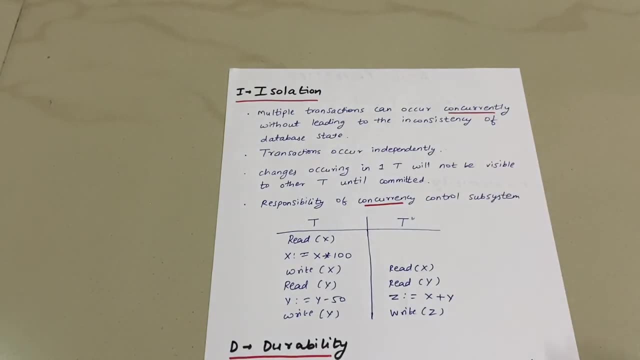 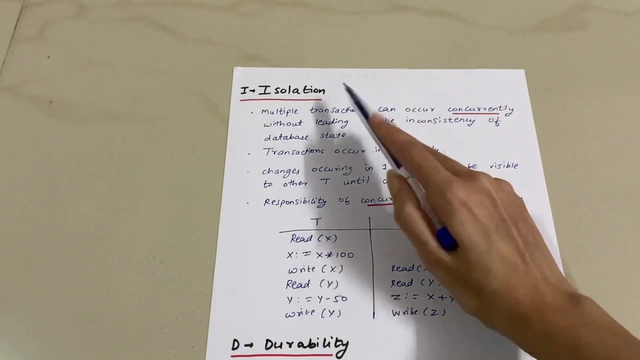 and all these transactions should occur independently. independently. this is what isolation means. so if I am, if I am withdrawing some money, it shouldn't affect someone else deduction of money, and if someone else is withdrawing money, it should be independent. so that is what isolation means. changes, changes. 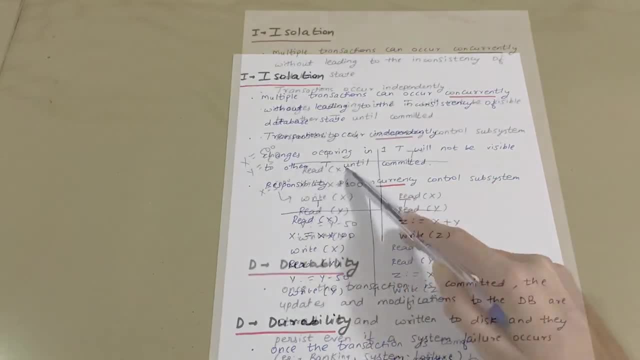 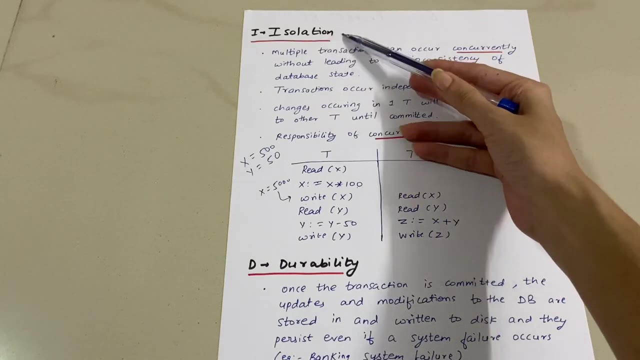 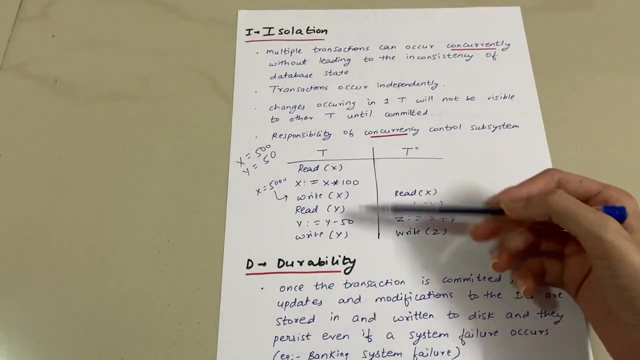 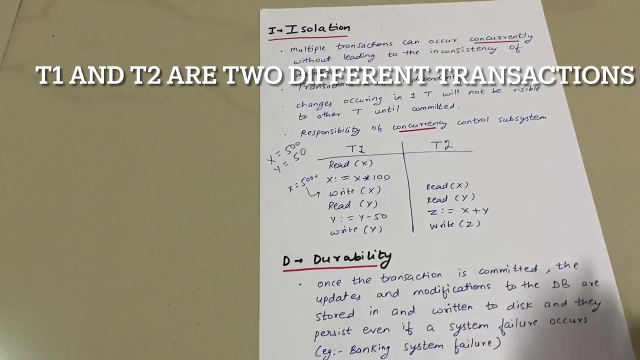 occurring in one transaction will not be visible to other. responsibility to to manage this property, to manage isolation property is of concurrency control substance, it subsystems. it is managed by concurrency control subsystems. so let's see an example. so there are two transactions, t1 and t2. so what are they doing? let's see. so let's consider X as 500 and Y as 50. so 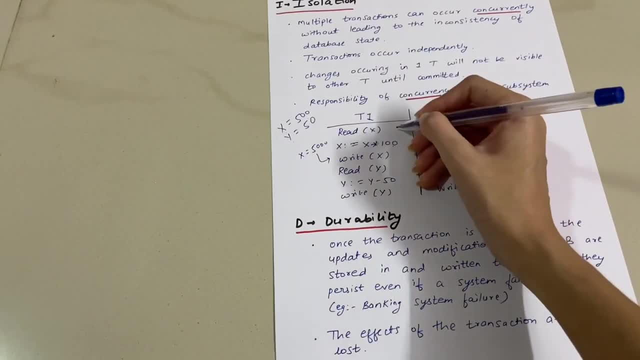 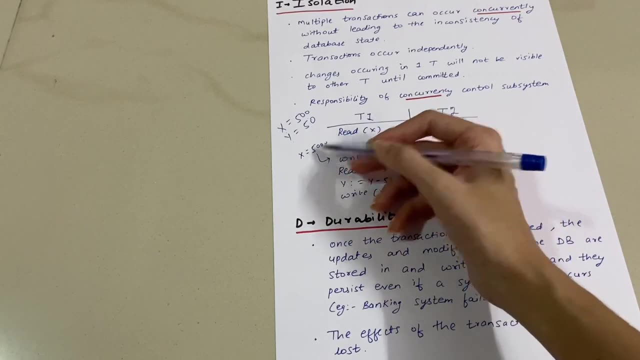 what t1 is doing is it will read X, so it will read X as 500, and then it will change the value of X to X. is X is equal to X into 500, so X will become 5,000. then it will write X, so it will write it into the memory, so X will become 5,000. 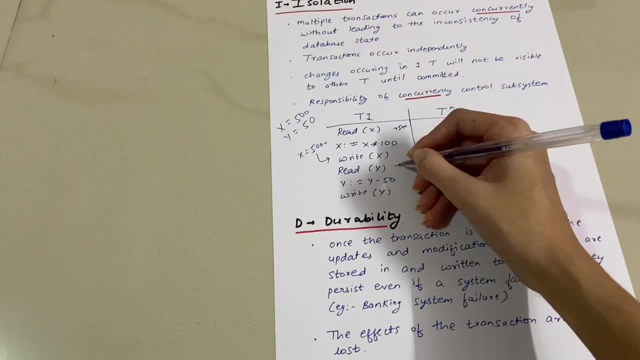 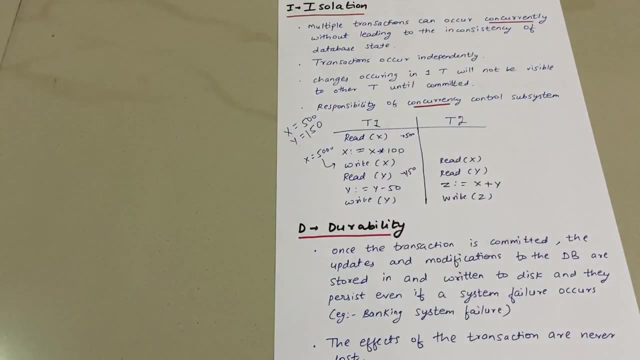 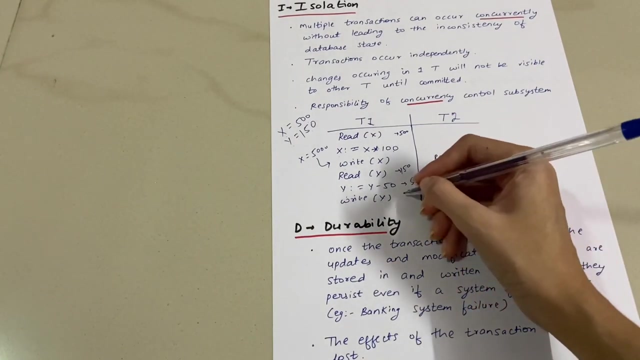 okay, then we will read Y, so Y is 50. sorry, let's consider Y as 150. okay, so it's reading Y as 150. then Y is equal to Y minus 50 means Y will become 50 and then we will write the value of Y as 50, so this will: 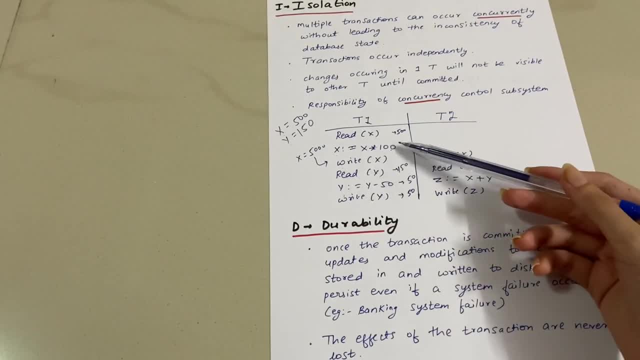 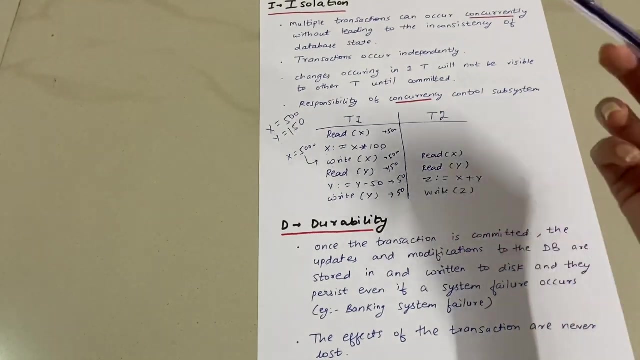 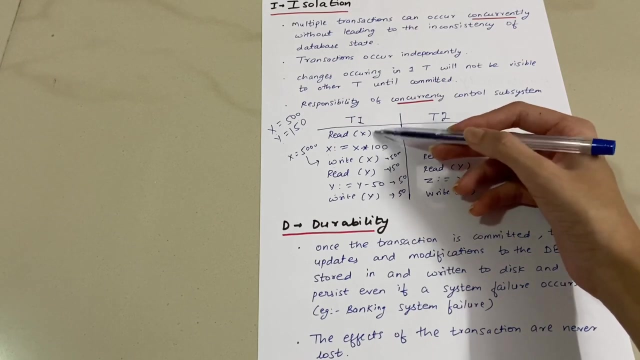 be the last value. so at the end of it, X will have the value 5,000 and Y will have the value 50. okay, okay, but if isolation is not there, what does isolation mean? is, for example, the X? the value of X will be Eurot until be 500. 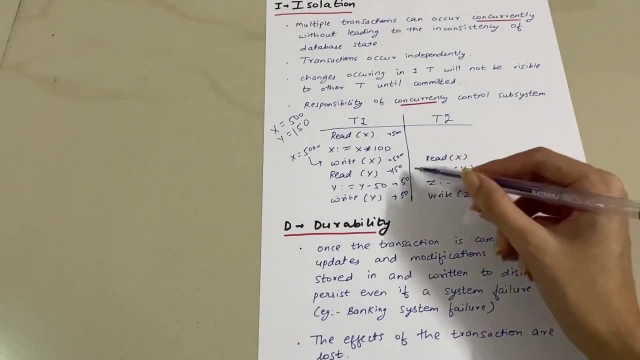 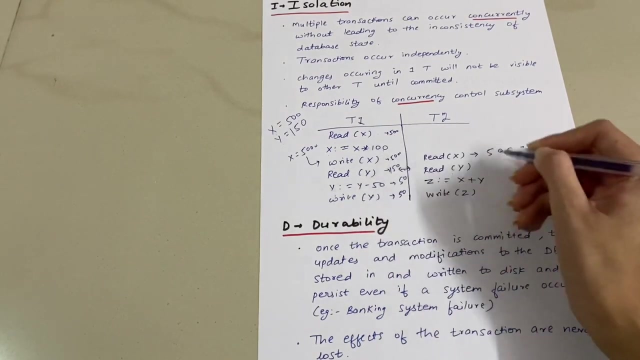 your Eurot will become 5000, but at the same time, if t2 is also reading it, okay. so here, if it's, it's reading it, so it will become 5000, okay. and here it will read value Y, but over here the value of Y, isition. 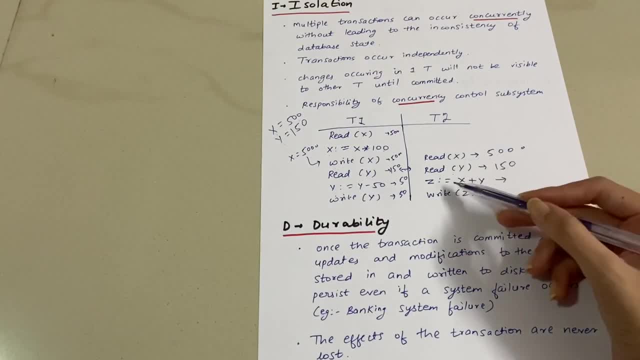 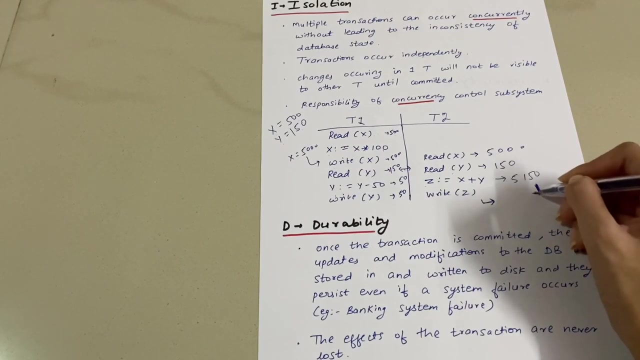 150 and then, and then the value of z will become 5150 and at the end of it, at the end of it, if you see, the value for y is different over here. the value of y which t2 is considering is different. t2 is considering y as 150. 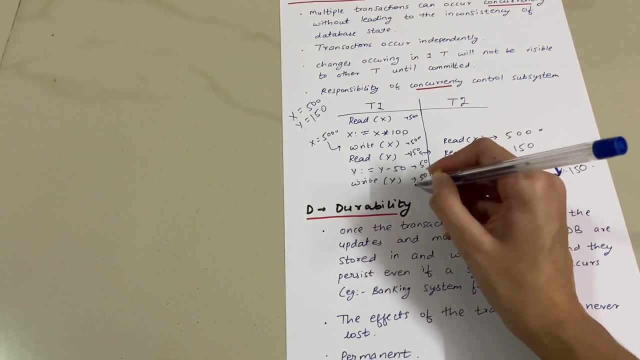 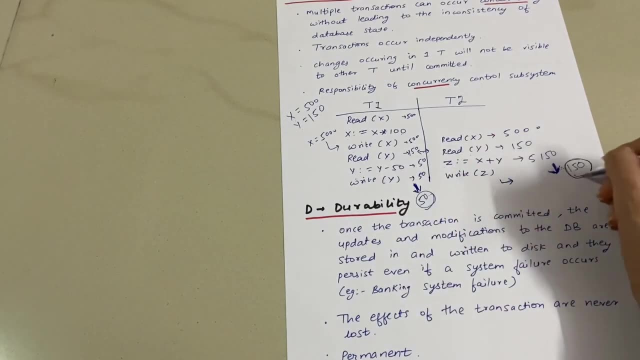 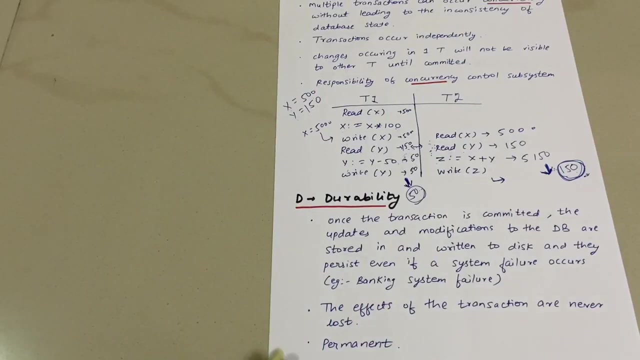 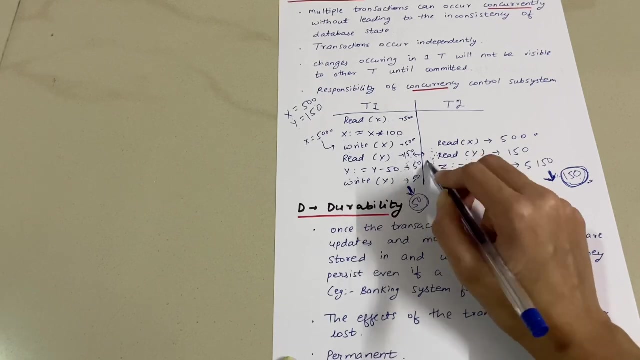 50, correct, but the value of y has been changed by t1 and it is 50, so there is inconsistency again. why is this happening? because both of these are interfering with each other. the values are being interfered, sorry so. so isolation. so transactions should follow this property called isolation. so t1, t1.